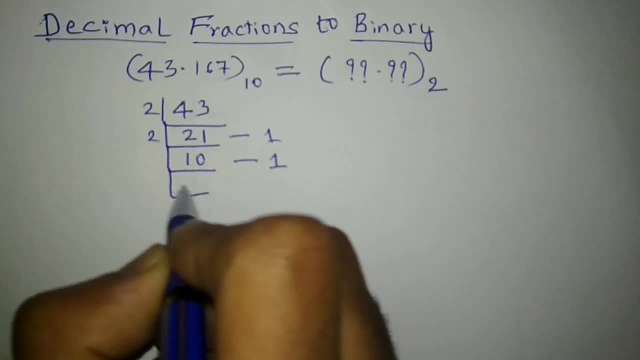 And the remainder is 1.. Similarly, I would divide this again by 2.. 2.5. It is 10. And the remainder is 0.. Next, 2.2.. It is 4. And the remainder is 1.. 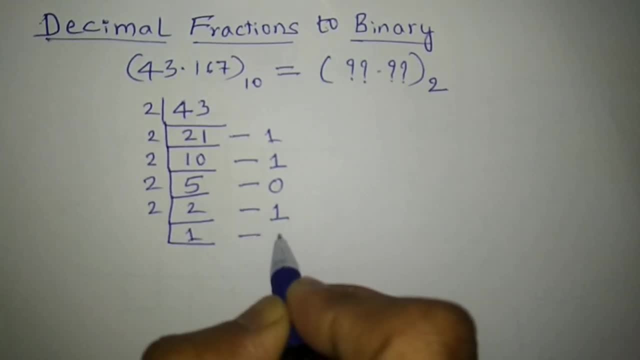 And lastly, 2.1.2.. And the remainder is 0.. So this is what its binary equivalent of integer part, That is 1.0.. I would have to go in this way. So that is 1.0.. 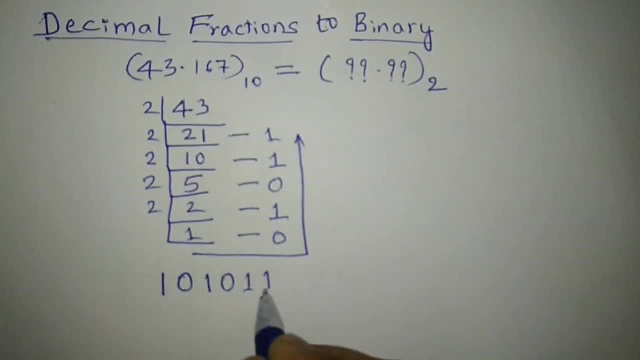 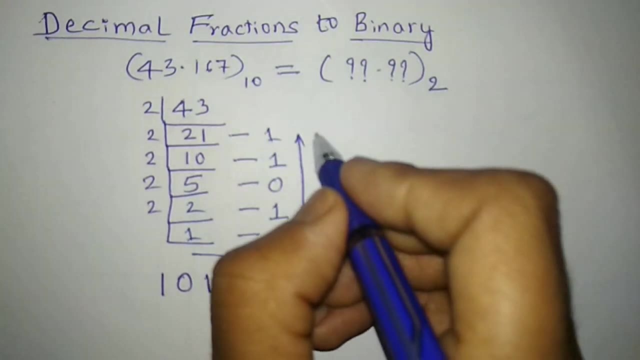 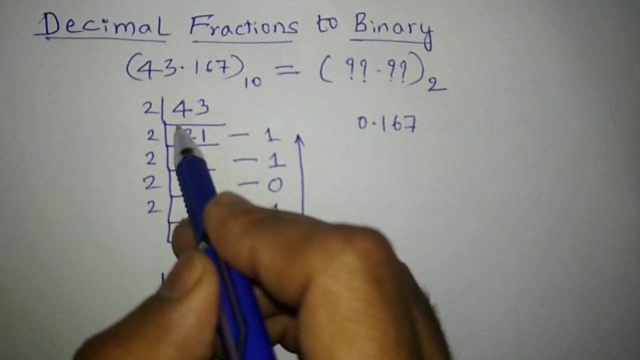 So that is 1.0.. 1.0.. 1.1.. So what is equivalent of fraction? I yet to need to find that one, So 0.67.. So the way I have divided the integer part successively by 2.. 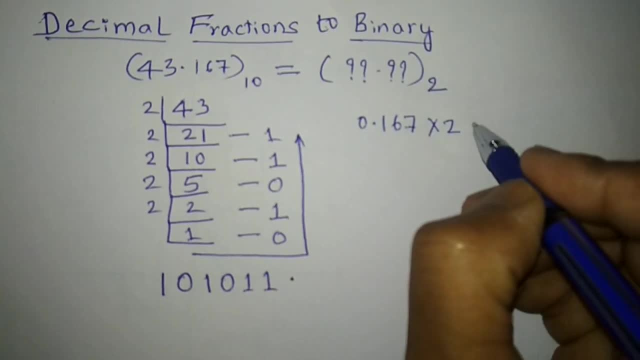 Here. I would multiply this successively by 2.. And let me see what do I get. So if I multiply 0.167 with 2., I am going to get 0.334.. So this is what its equivalent in binary. 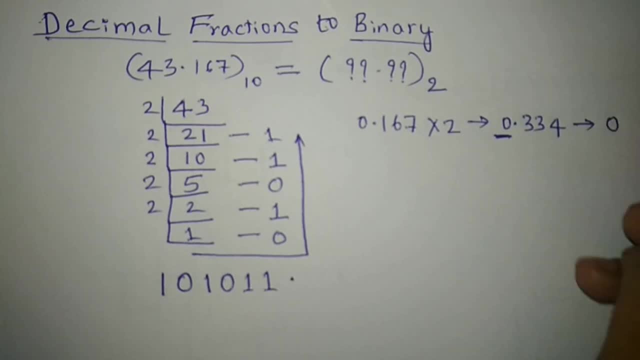 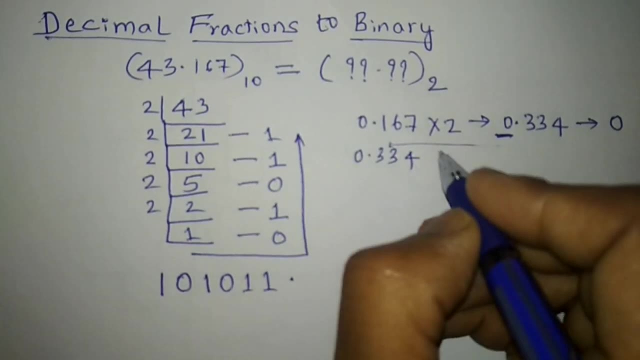 Whatever I get here, that is, I take it as 0.. So next what I do is I will consider 0.334.. So this is the answer I got. I would consider it here And I would multiply that with 2.. 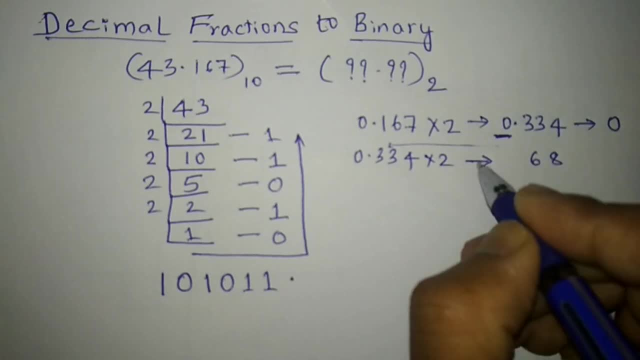 So it is 2.48.. 2.36. And 2.36.. So it is going to be 0.668.. So integer part is 0.. So I would consider that as its binary equivalent. 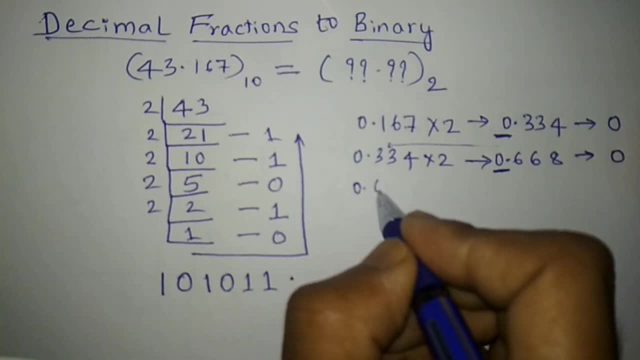 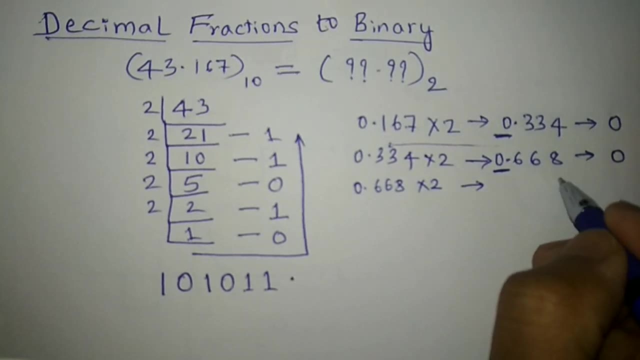 It is 0.. So next I would consider 0.668.. 0.668.. I would multiply this with 2.. So what do I get? It is 8 to the 16 with a carry 1.. 6 to the 12 with carry 1.. 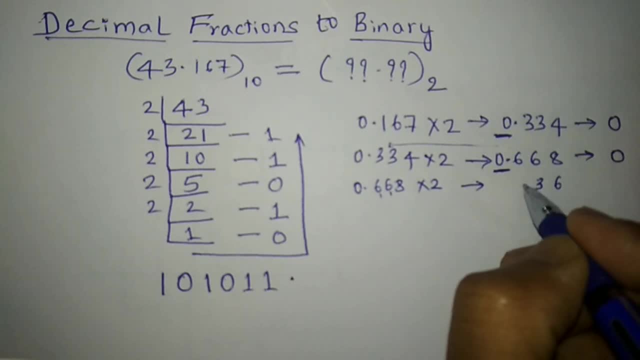 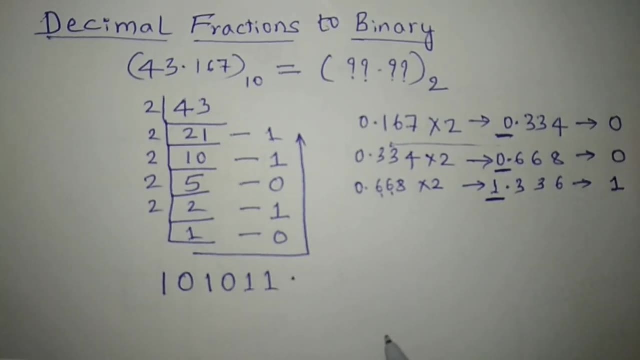 It is 13.. Carry 1 again 6 to the 12. 13. So I would get this as 1.. So its binary equivalent Here I would write it as 1.. So next, what I would do is I would consider only this fraction part.